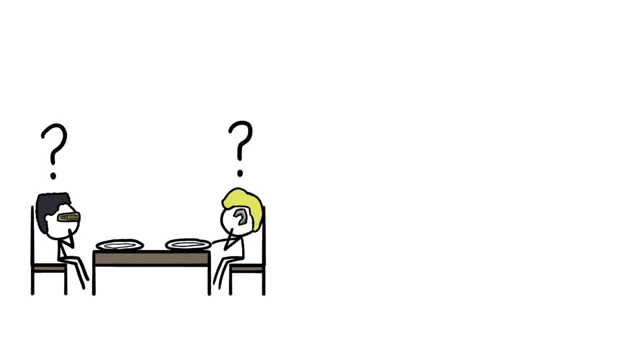 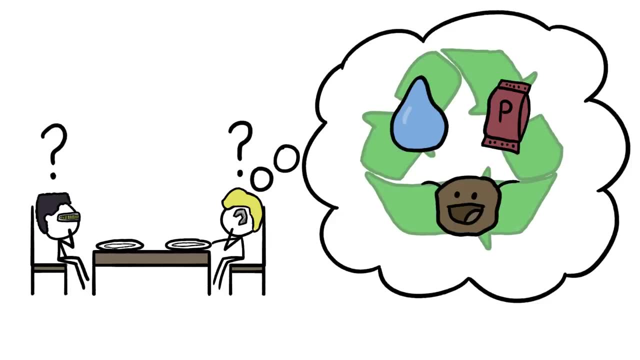 years. So what are future humans going to do about dinner? One possibility is to switch to a food-making system where resources get recycled rather than depleted. Radical as it sounds, this kind of system already exists all around us in nature, where sunlight is the only major. 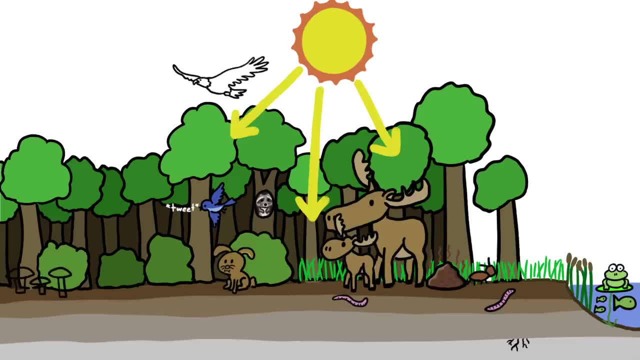 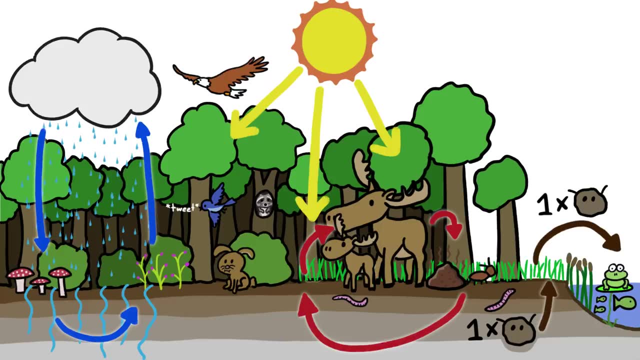 energy input and ecosystems comprised of many different coexisting plants and critters cycle nutrients and water within the system or use water to produce food. So what are we going to do? We have started taking some cues from natural ecosystems, like interspersing crops with trees. 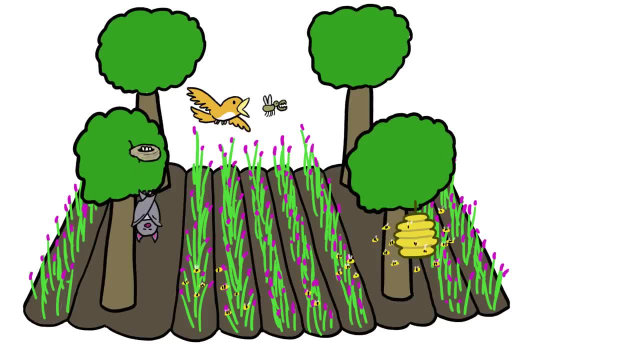 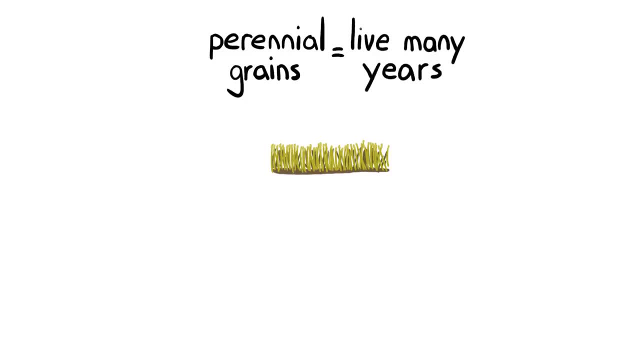 to encourage a healthy habitat for pollinators and pest controllers, and by changing the crops themselves. For example, we've begun to develop perennial forms of wheat, rice and other grains that can live through many harvests, unlike traditional grains, which we have to plow and 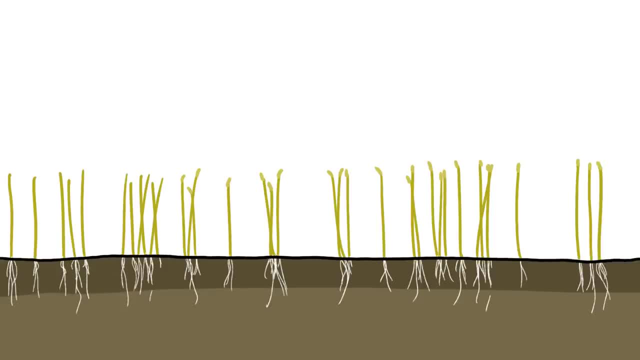 replant every year. The idea is to eventually grow the new grains alongside a variety of other long-lived plants. So what are we going to do? Well, we're going to start with a variety of crops and vegetables and self-sustaining ecosystems that keep hold of soil water. 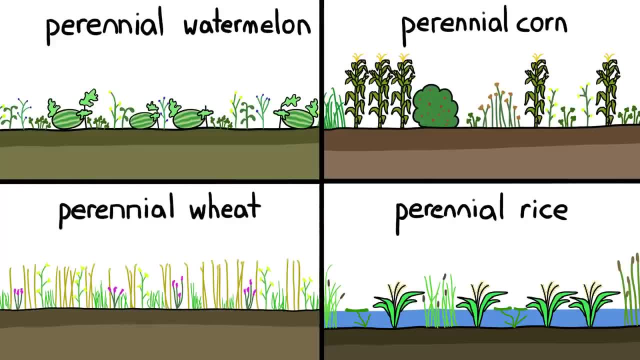 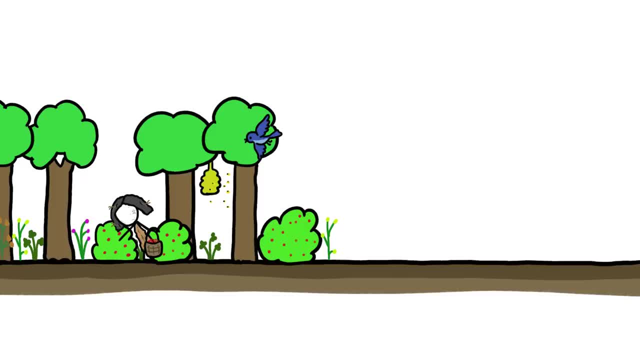 and nutrients. If we could manage to do this for all of our food, it would be qualitatively different from any other way. humans have grown food on a large scale, Not quite hunting and gathering, not plant-harvest repeat, but a sort of futuristic blend between the two. 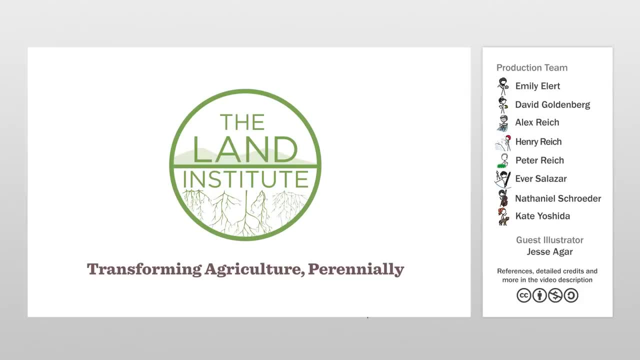 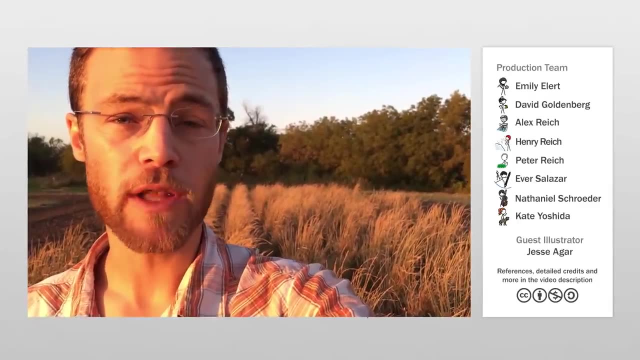 Hey there, I'm Alex. I'm here visiting the Land Institute, the sponsor of this video. They're creating a new form of agriculture. The Land Institute's goal is to develop a variety of agricultural ecosystems in order to help feed the world's population with fewer environmental impacts. Here at the Land Institute, plant breeders. 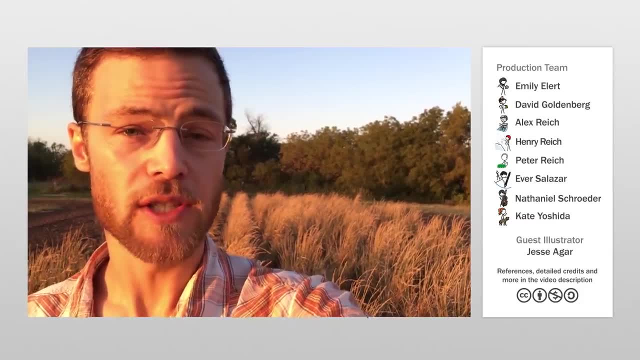 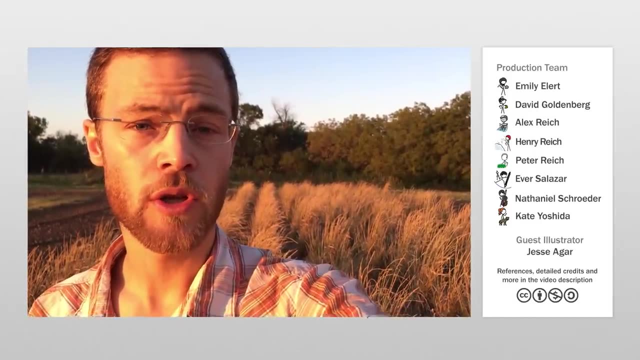 and ecologists are developing perennial grains, legumes and oilseeds like these behind me. The goal is to grow them in ecologically functional and diverse mixtures called polycultures. To learn more about how the Land Institute's perennial polycultures could help revolutionize 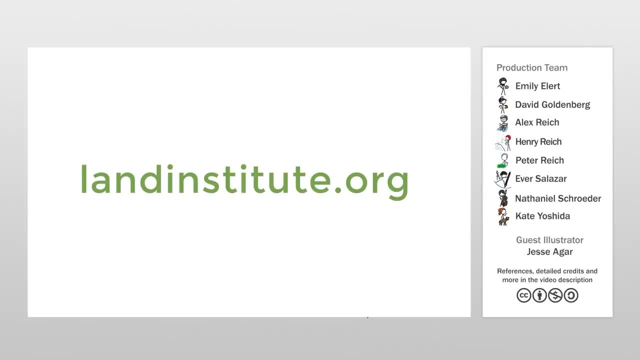 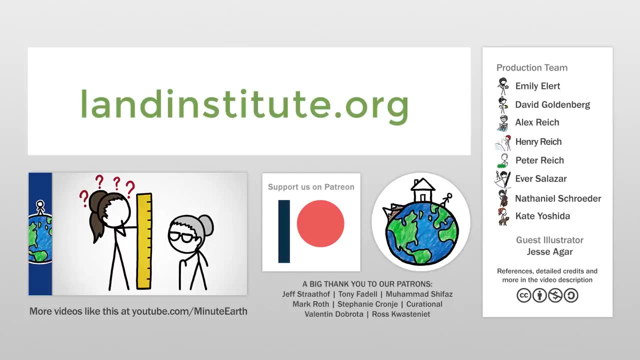 agriculture or to support their work, visit landinstituteorg. The Land Institute is a proud sponsor of this video.